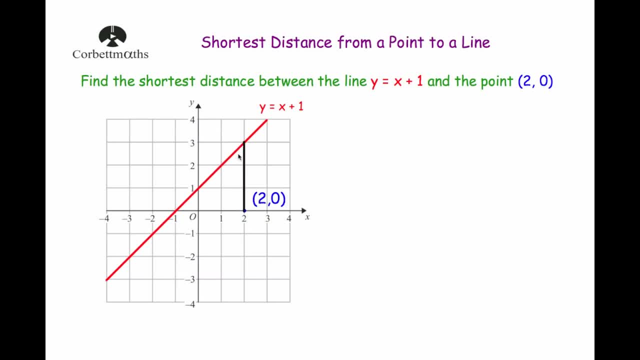 line. Now, if you were to go straight up from the point 2, 0 to the line, you can see, it would be 1,, 2, 3 units. If you were to go horizontally from the point to the line again, 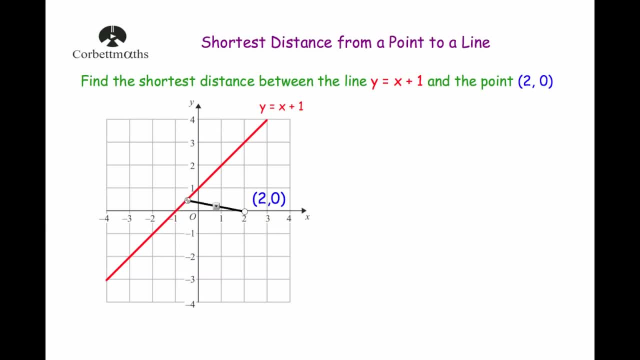 you would see it would be 1,, 2,, 3 units. But as you move across diagonally, like so you can see, the line gets much shorter. And it's at its shortest whenever the line- this black line- is at right angles or is perpendicular to the red line. So in other words, it's perpendicular. 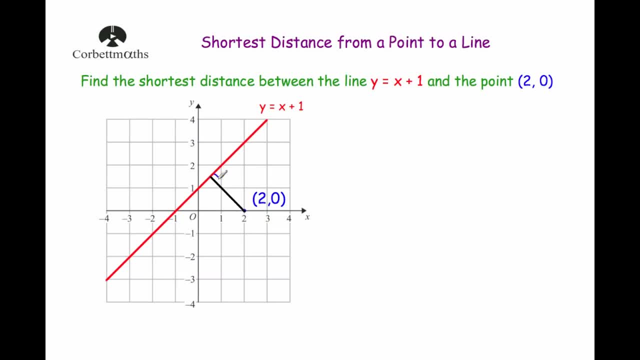 to the line you're given in the question. So if we want to find the shortest distance from a point to a line, there's three steps. we've got to follow Number one: we've got to find the equation of the perpendicular line to the line given. 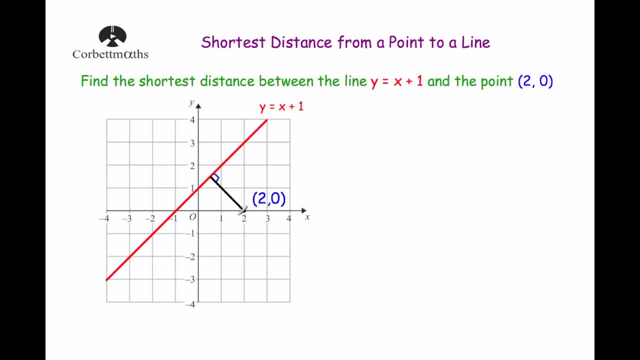 That passes through the point that you're given in the question. Step two: you want to find where the line that you're given in the question and your perpendicular line, where they intersect, And in other words, you need to find this point here, the coordinates. 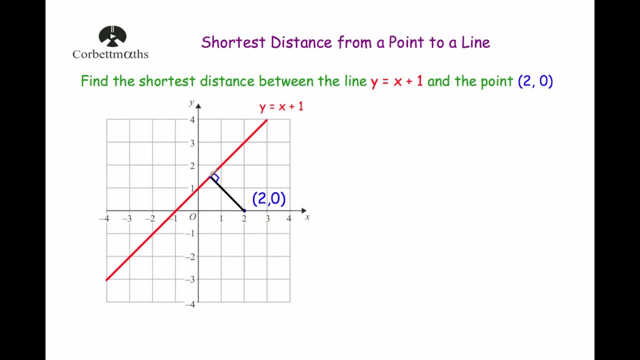 for that point. And the last step is: you're going to use Pythagoras to find the length of this diagonal, Because, as you can see, you've got a right angle triangle. If you use Pythagoras, you can find the length of this black line, And that would be the shortest. 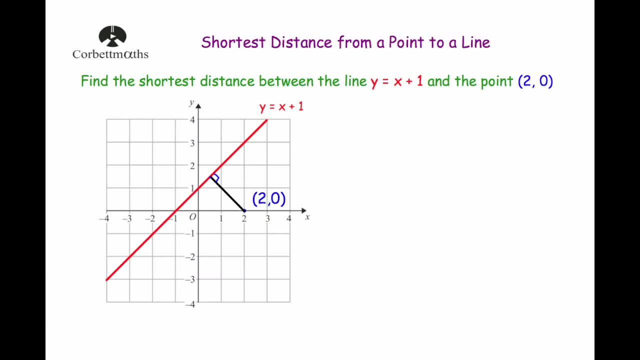 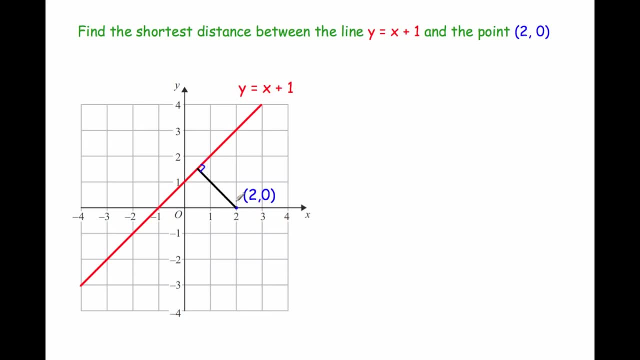 distance from the point to the line. Okay, let's have a look at that now. So here we've got the same question And we're just going to follow those steps. So step one: we've got this perpendicular line. Let's find this equation. So the equation: 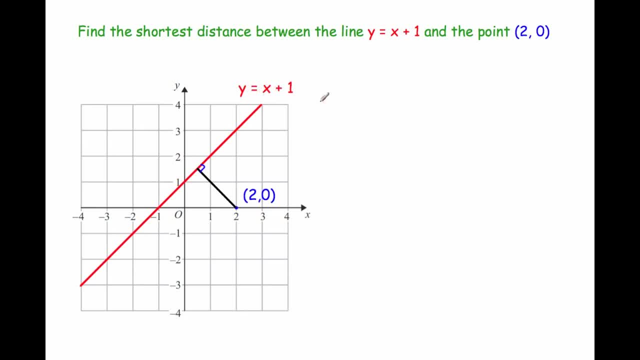 of the line that we're given is: y equals x plus 1.. So a perpendicular line or the gradient will have the negative reciprocal. So if the gradient of this one's 1,, the gradient of this one will be minus 1, or we call it minus x instead of writing minus 1x and plus c. 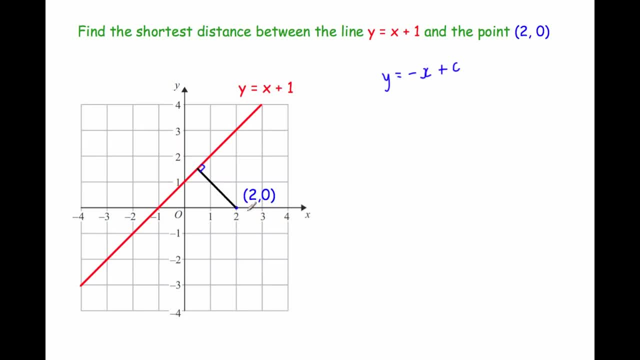 Let's find c, the y intercept of this black line. So we know that it passes through the point given to 0. And that's in the format x and y. So if we substitute these in we can get the same thing. 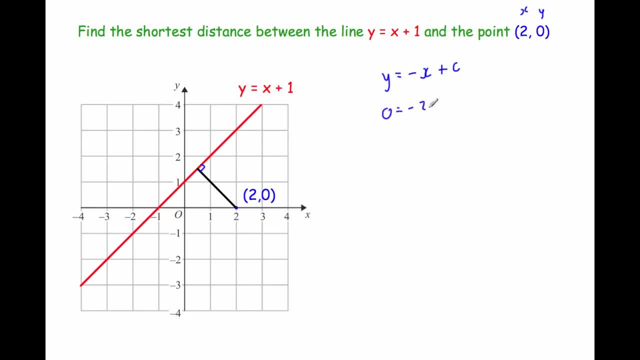 So 0 equals minus 2 plus c, So c equals 2.. So the equation of this black line is: y equals minus x plus 2.. So that's the first step done. We've found the equation of the black line, or the equation of that shortest line. And now what we're going to do is we want to find 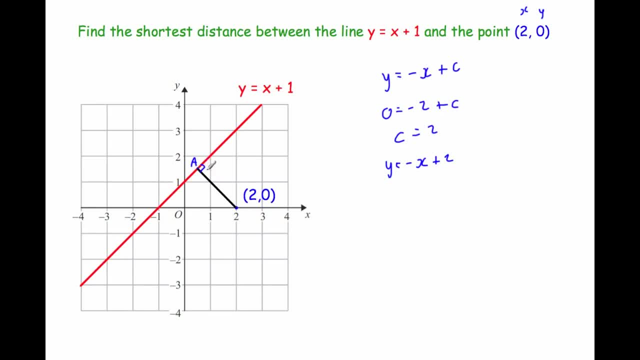 this point here. Let's call it a. okay, this point And the coordinates of a can be found by considering simultaneous equations. We've got this red line, which is y equals x plus 1.. We've got this black line, which equation is y equals minus x plus 2, to find what they 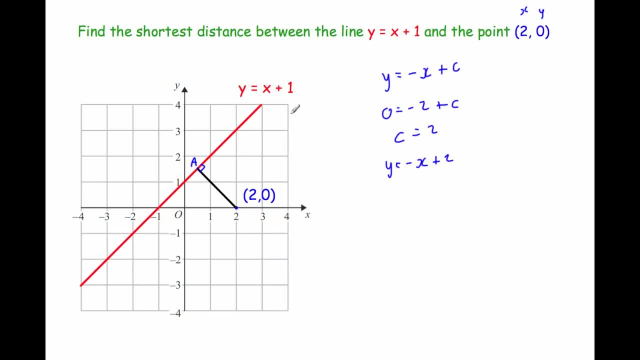 intersect to each other. Well, I would probably use substitutions of replacing this y with the x plus 1.. As you get x plus 1 equals minus 2, or so minus x plus 2.. And if we solve this, adding x to both sides, we're going to get 2x plus 1 equals 2.. And minusing one from. 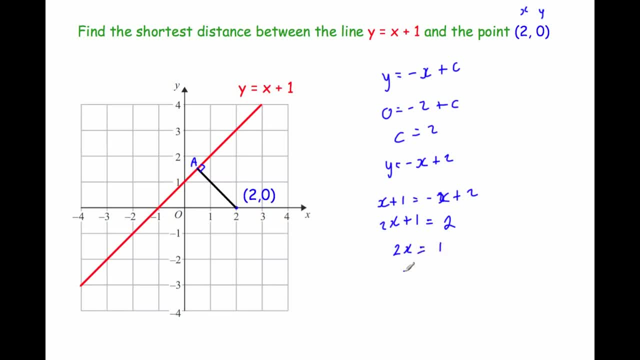 both sides, we're going to get 2x equals 1.. And dividing by 2, we're going to get 1 plus x. we get x is equal to 0.5. so this point- here it's x coordinate- is 0.5. now we need to find what the 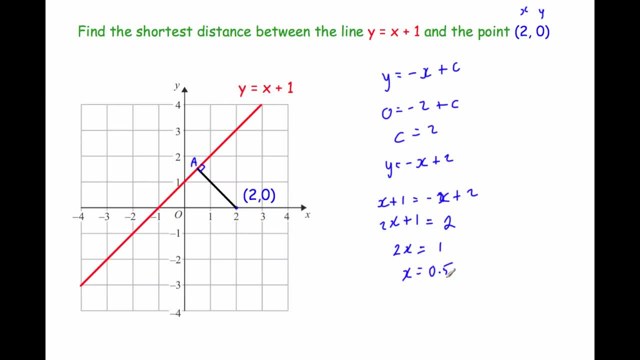 height of it is well the height. well, we can substitute this 0.5 into either one of these two. like you can with simultaneous equations, i'm going to substitute the 0.5 into this one. so y equals 0.5 plus 1, y equals 1.5. so this point a has the coordinates 0.5. 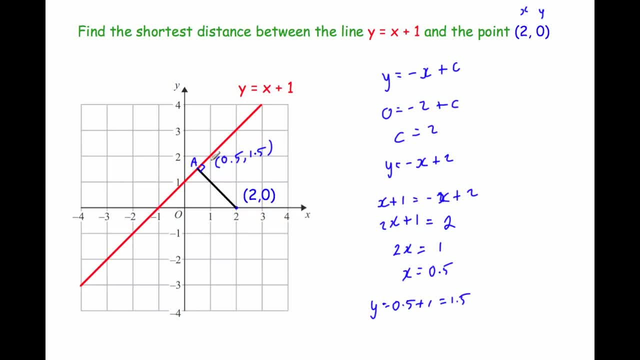 0.5, 1.5, and that's it. and our last step is to find the distance between this point a, which is 0.5, 1.5, and the point we're given in the question, which was 2, 0. there's an equation for that, that is um. this equation, here, the square roots of brackets x2. 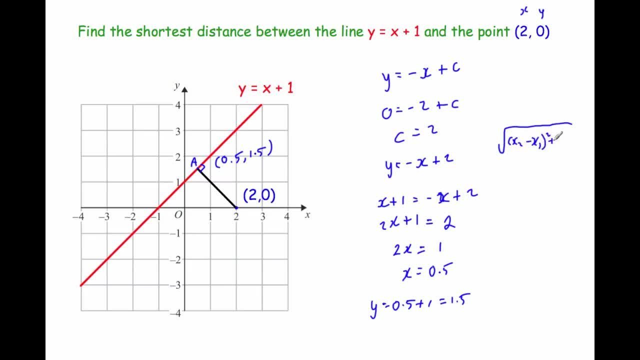 minus x1 squared, plus brackets, y2 minus y1 squared and you can just plug those values in, so you could call this one x1 and this one y1 and this one x2 and this one y2 and plug them in and work it out. 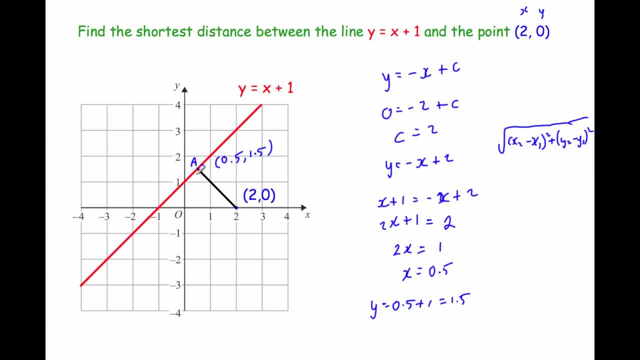 or the way i prefer to do is just to consider a right angle triangle and use Pythagoras because, as you can see, if you just go across, down and across, you've got this right angle triangle and this point- here it was 0.5 and it goes across to 2, so that was 0.5, and across the two sets, if 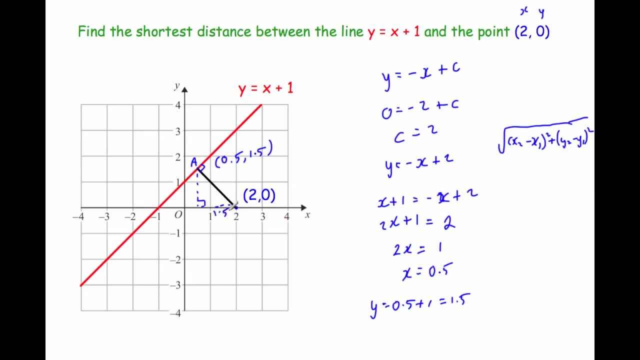 you go across, it's got a length here of 1.5. i'm actually just going to sketch it this out. that's the point a, that's the point 2: 0 and we've got, we've seen here that if we just go across it's 1.5 across. and again this has got a height. this point here is a height of 0 and if we 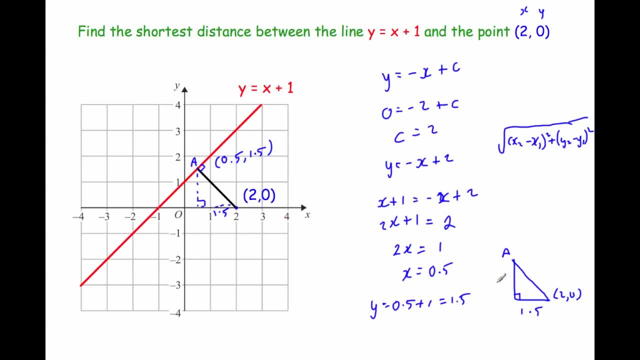 go upwards to here, it's got a height of 1.5. so again this would be 1.5, and we could just use Pythagoras on this. so let's just work that out. so a squared plus b squared equals c squared, so that would give us 1.5 squared plus. 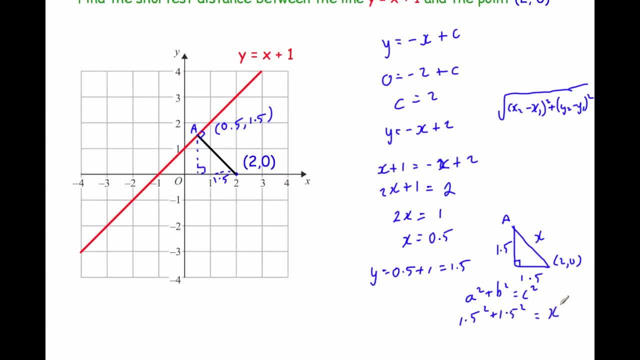 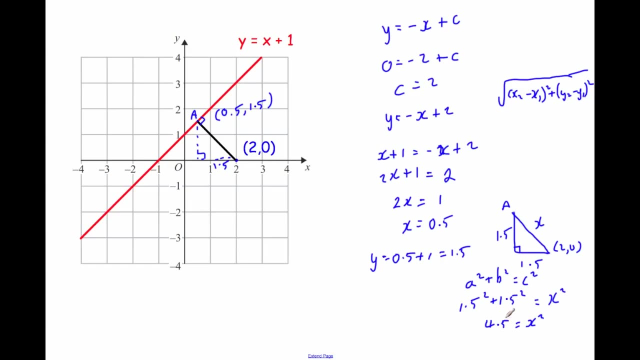 1.5 squared equals x squared. 1.5 squared plus 1.5 squared, that is 4.5. you can test that on your calculator if you wish, and now you just need to square root that, so the square root of 4.5 would be equal to x equals 2.12132, and so that's the shortest distance. so the shortest. 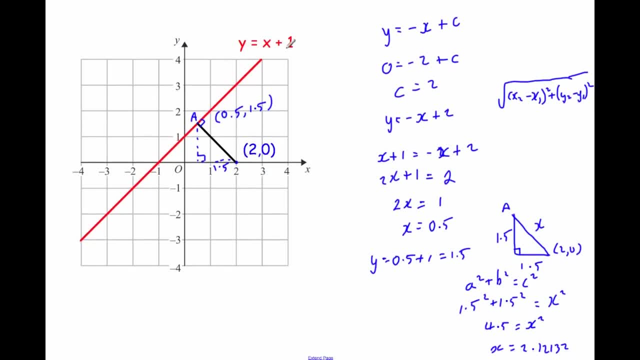 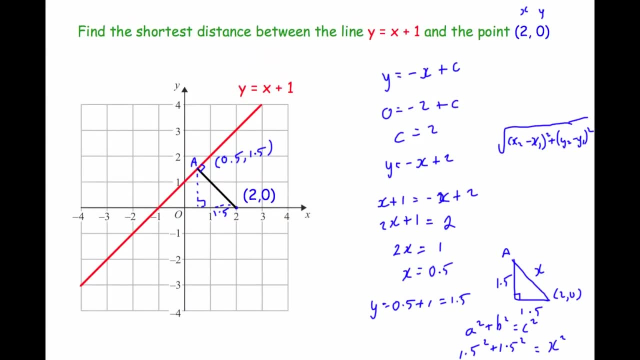 distance from the point 2: 0 to the line equals x plus 1 is 2.12132, and that's it so, and that's it so. to find the distance between a point and a line, there's just three steps you follow. find the equation of the perpendicular line that. 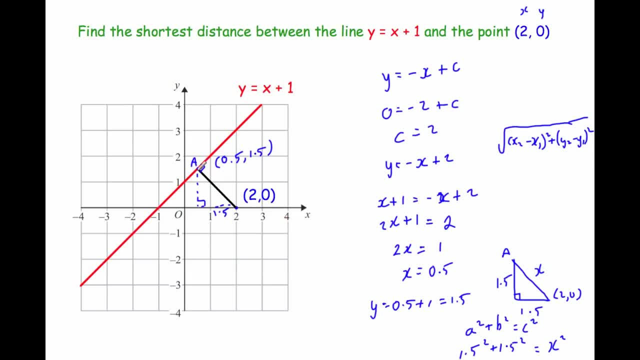 passes through that point to the line that you're given, find the coordinates of where those lines intersect and then use Pythagoras to find the length of that line segment. and let me just show you, on another question, how it attempted. i'm not going to do the whole question, just going to show. 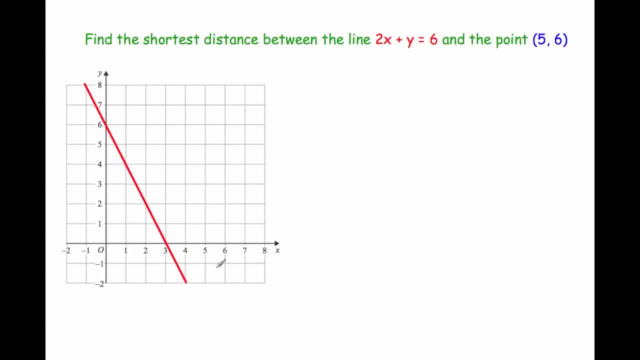 you what we're doing this time. we've got this red line here, we've got the line 2x plus y equals 6, and we've been asked to find the shortest distance between that three.5 six. that is the point here. so what you would do is again draw the perpendicular line. 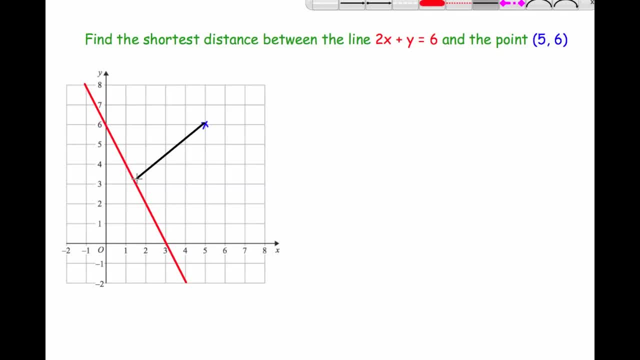 again. this is just. this is just gonna be a very rough sketch here. okay, so there's a perpendicular line, ish to the point given and, and then the steps would be. they would be a little bit shifty, so that will do that. there will be a couple apartment. so this is just a last to have a presentation of. 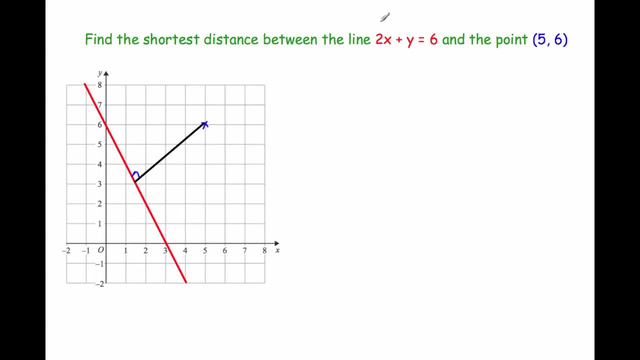 be find the equation of this black line. so the line that we were given was 2x plus y equals 6. well, I would make y the subject. so y equals minus 2x plus 6. so that's this line: y equals minus 2x. 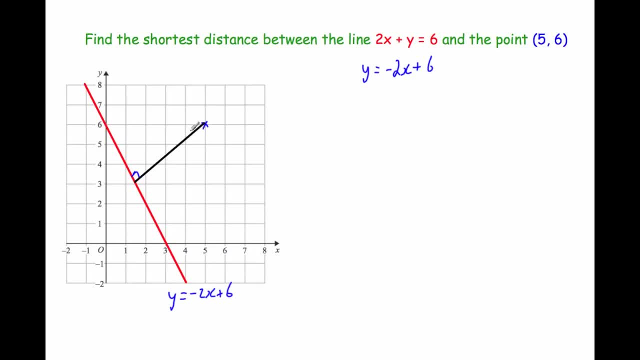 plus 6, this one. here the equation would be where the gradient is the negative reciprocal. so the negative reciprocal of 2 is a half. so this line would be: y equals a half, x plus c. I would actually I'm just going to carry on and do this question just because I'm nearly finished it. okay, so at 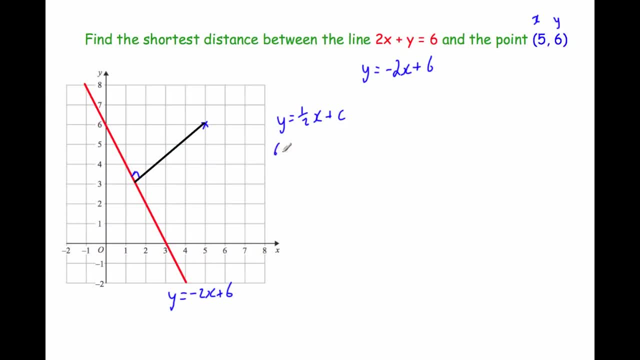 this point. here it's x and y, so plugging these in 6 equals a half of 5, that's 2.5 plus c. c then equals 3.5. so the equation of the black line is: y equals a half x plus 5. 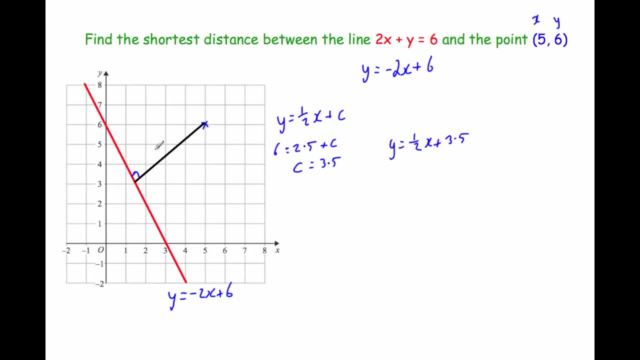 3.5. as you can see, my sketch isn't very good in terms of where that black line is. it's more probably up this way. anyway, that's step one was to find the equation of the black line. step two is to find where the black line and the red line intersect, in other words where the 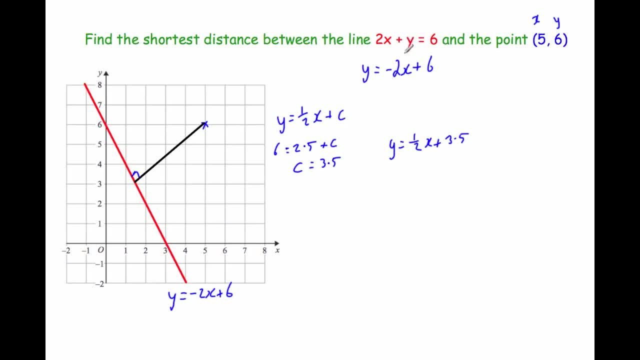 perpendicular and the line given in the question meet each other, so let's solve that. so we've got y equals a half x plus 3.5, and we had y equals minus 2x plus 6. so if we equate them, so minus 2x. 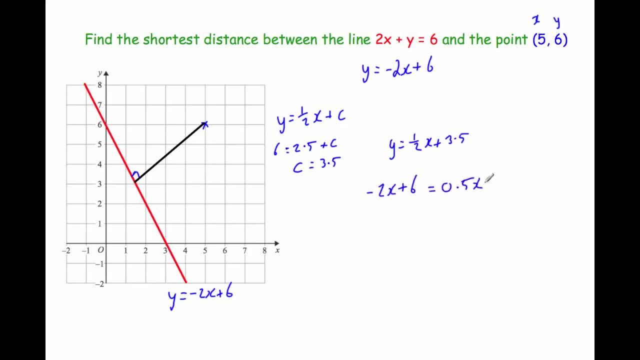 plus 6 equals 0.5 x plus 3.5. solving this, I'm just going to bring the 2x over here to get 6 equals 2.5 x plus 3.5. tick the 3.5 off will give me 2.5 equals 2.5 x, so x equals 1. okay, that's cool. 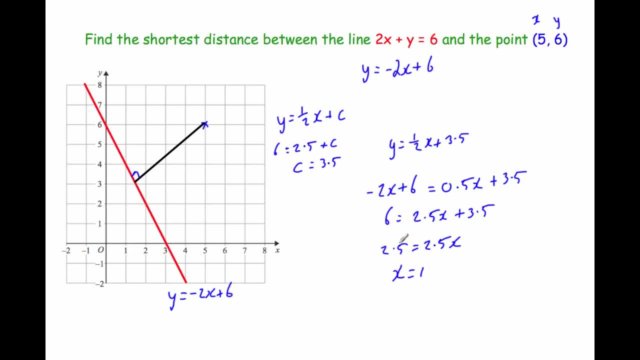 plugging that back in to one of these two should get the same, no matter which one you use. I'm going to use the top one here. minus 2 times 1 is minus 2 plus 6 is 4. so y equals 4. so the point.